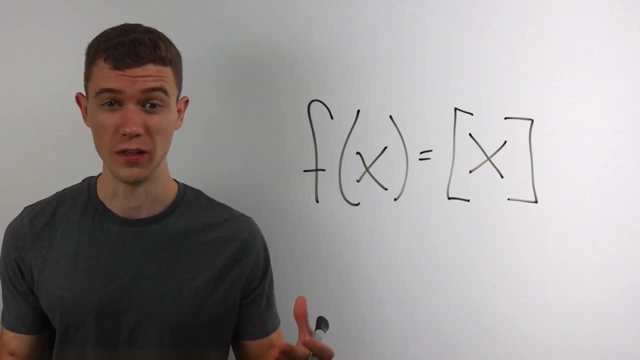 This is the so-called greatest integer function, And what does it do? Well, you might have guessed, it outputs the greatest integer of x. Now, I've seen it denoted like this. I've also seen a double bracket before And I've also seen only like these lower brackets, So sometimes the greatest. 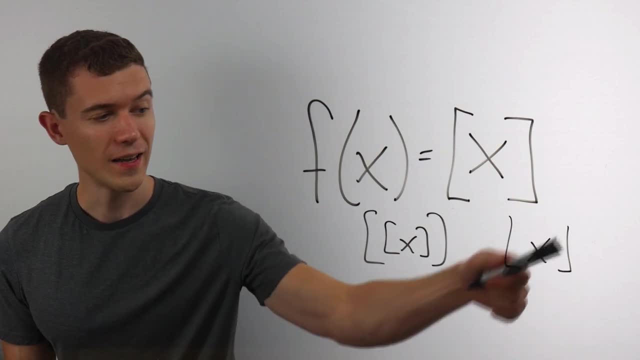 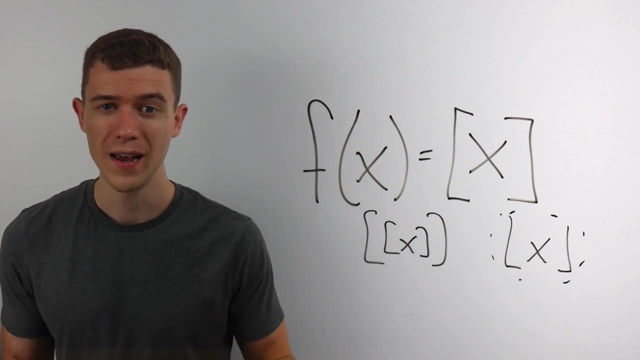 integer function is called the floor function, And this one is usually what people mean when they say the floor function. I guess the little lower brackets make a floor. And what does this thing do? Well, as we said, it's the greatest integer function. it outputs the greatest integer. 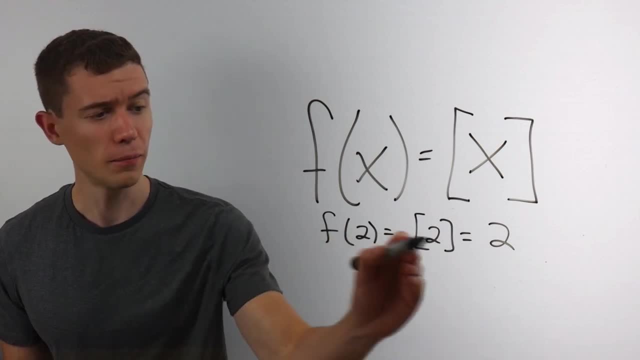 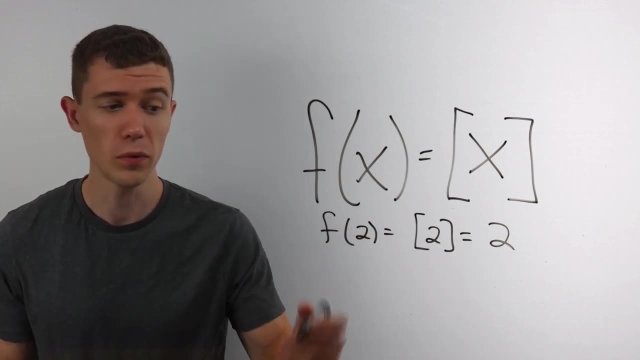 less than or equal to the input. So if I plug in to the greatest integer less than or equal to two is to remember integers are whole numbers. But if I put in something like f of 2.1, what's the greatest integer less than or equal to? 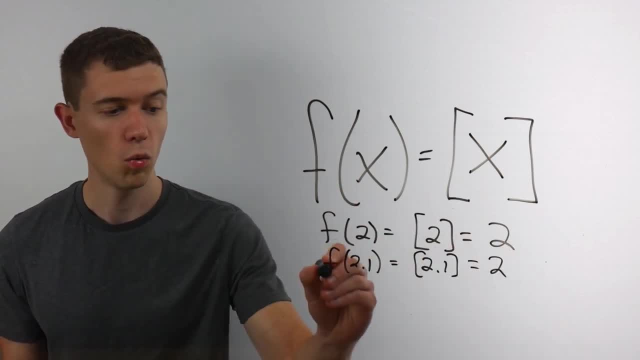 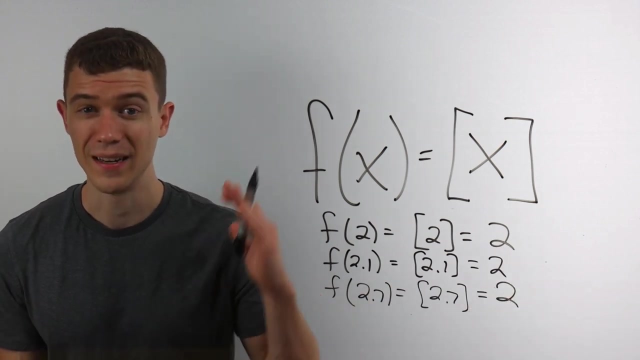 2.1, it's still just two. What about if I plug in 2.7?? What's the greatest integer? less than or equal to 2.7, it's still two. right, we don't round up. basically, we're always rounding down. 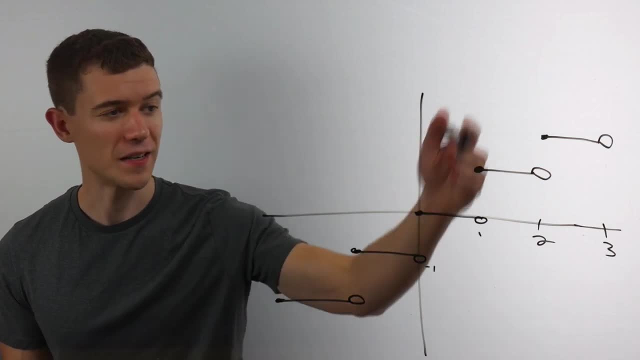 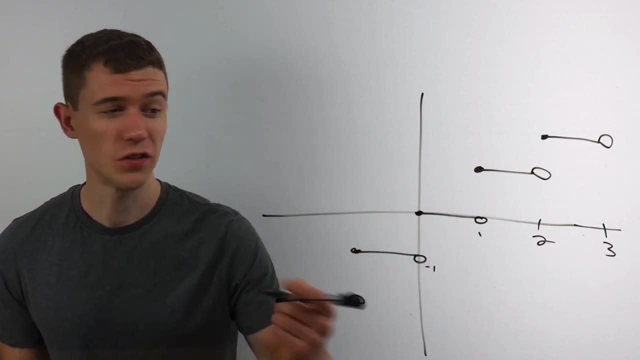 That's the idea. Here's the graph of it. you can see it kind of makes this staircase, So you might even call this a staircase function, But it works exactly the way we just described. If I plug in a two, it becomes a two. This is exactly what it looks like And, once again, you can see. 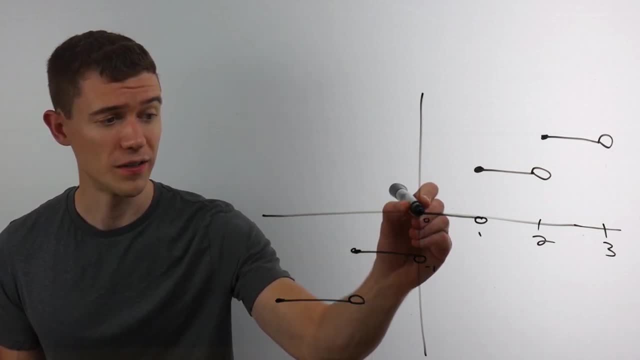 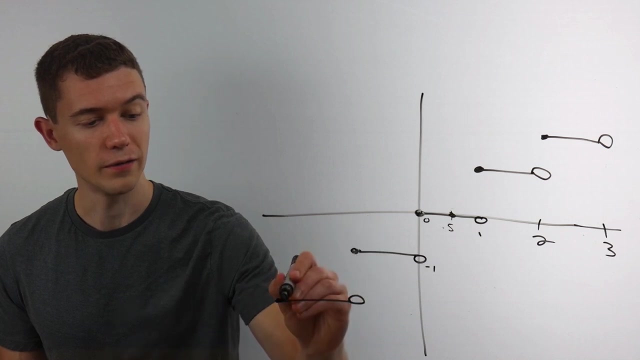 plugging zero. what's the greatest integer less than or equal to zero? Well, the output would be zero, And any number in between zero and one would also output zero. like if I plug in point five, I would round down to zero. Notice the closed circles on the left. 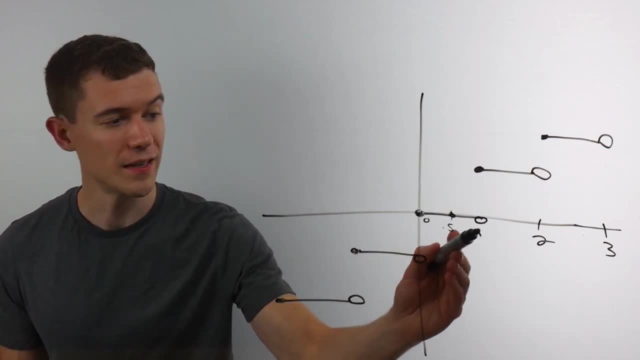 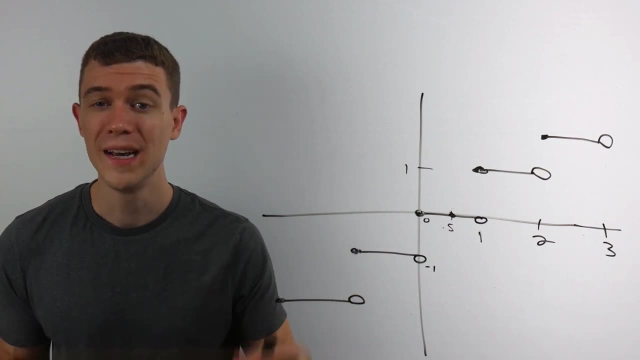 and the open circles on the right. That's because the greatest integer less than or equal to one is positive one. So this is the graph. it's a good thing to know in the situation where it comes up. But this was just a brief intro to the greatest integer function. I. hope you have a great day.